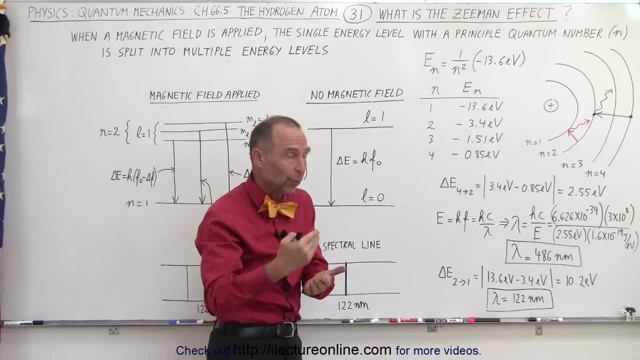 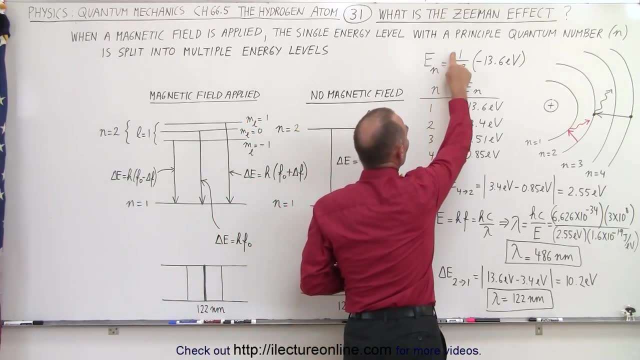 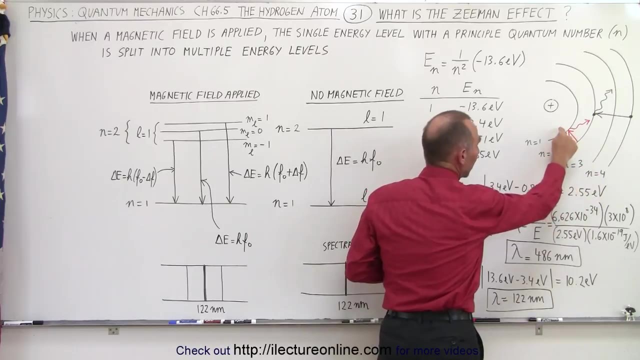 The way we can calculate what those photons are and what the frequency and wavelengths are is to know the difference in the energy levels. And the energy levels can be calculated using the equation of 1 over n squared times minus 13.6.. Electron volts minus 13.6 electron volts is the energy level of the innermost energy, where the principal quantum number n equals one. 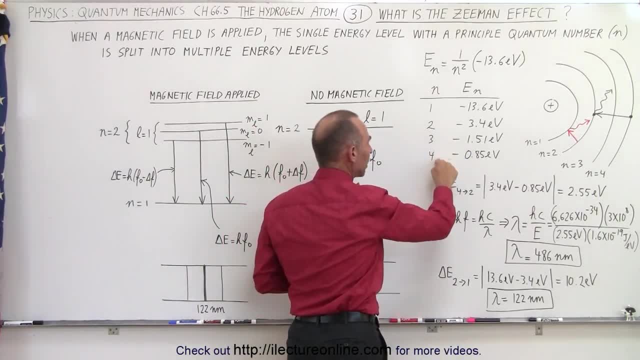 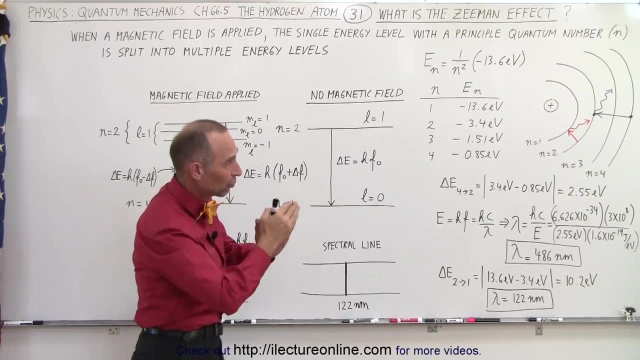 And so, therefore, at higher energy levels- n equals 2,, n equals 3,, n equals 4,- we can calculate the associated energy levels of those particular regions, And so, therefore, when electrons jump between those, they will then emit a photon that has an energy equal to the difference of those levels. 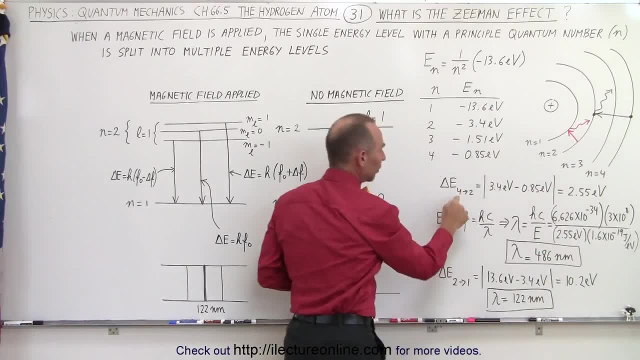 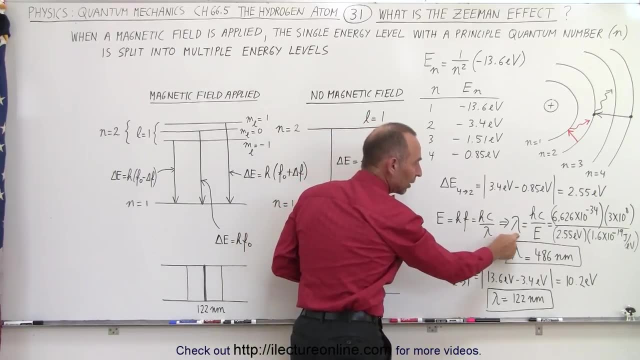 For example, when an electrons jumps for the 온, the photon will create an autumn energy which is equal to the difference of those levels. fourth level, down to the second level, the difference in the energy is 2.55 electron volts, and when we then calculate the wavelength of that photon, we can see that it's about 486 nanometers. 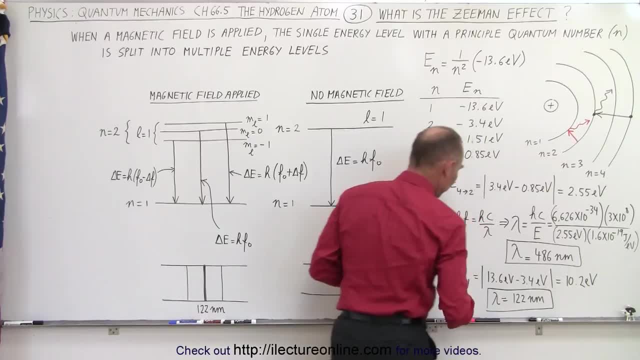 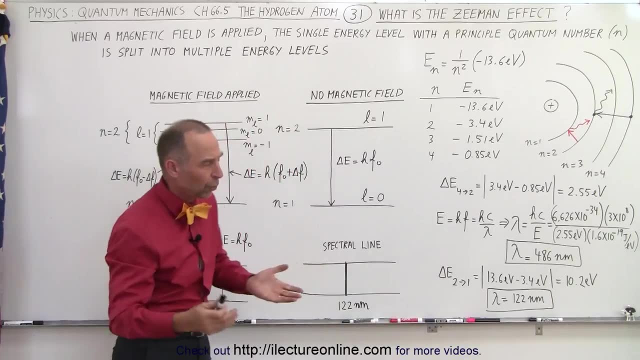 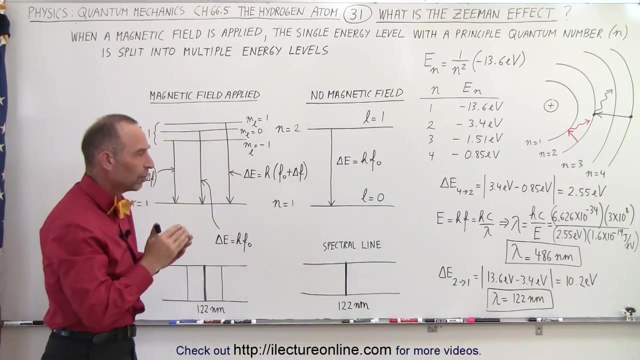 likewise, when electron jumps from the second level down to the first level, we can calculate the dissociation, dissociated wavelength of that photon: 122 nanometers, which of course would be a ultraviolet photon, where this was a visible light photon. so these, these spectrums, the 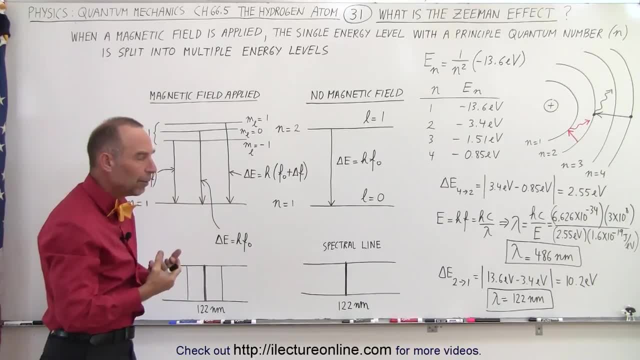 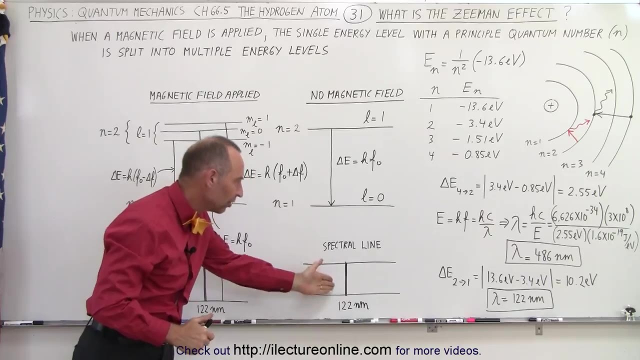 spectra of those jumps was was already discovered. but then something happens that was very strangely. when we took the hydrogen atoms and we subjected them to a magnetic field, we saw something different. we saw additional lines in the spectrum. so instead of seeing a single spectral line for that particular jump, we would see the same single line, but would see 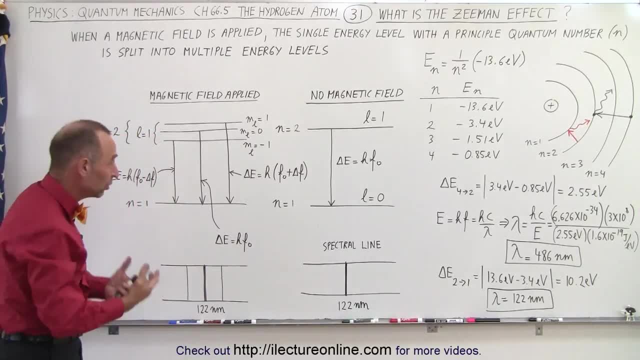 two additional lines, but on theζ additional lines. And the question was: why would we see two additional lines when a magnetic field was applied? And of course, if you saw the previous several videos, we realized then that the angle momentum of the orbiting electron can only have discrete directions And the 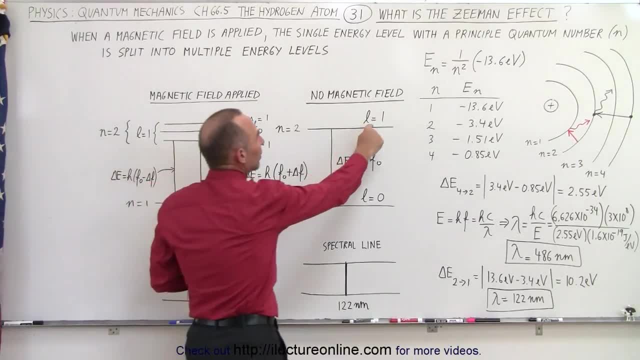 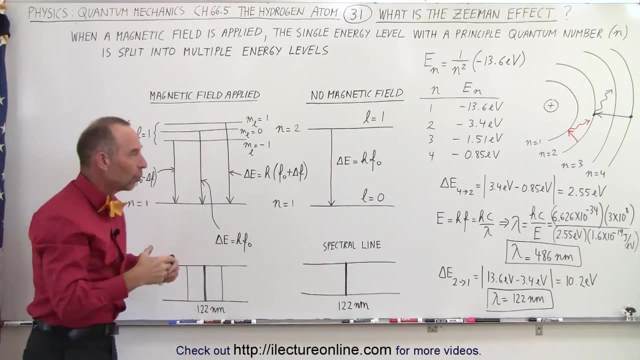 number of discrete directions are dependent upon L, which is the orbital quantum number. So when L is equal to one, there will be three m sub L possible values, which means when L equals one there are three different orientations of the angle, momentum And the energies of. 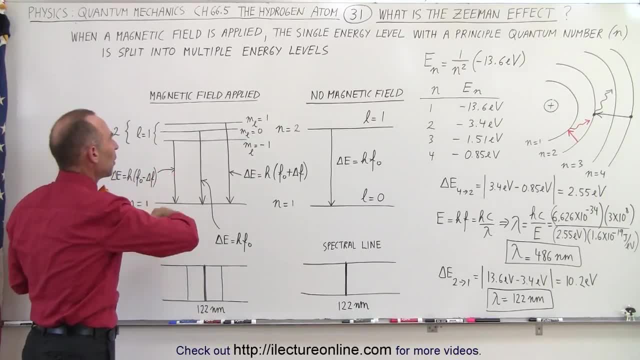 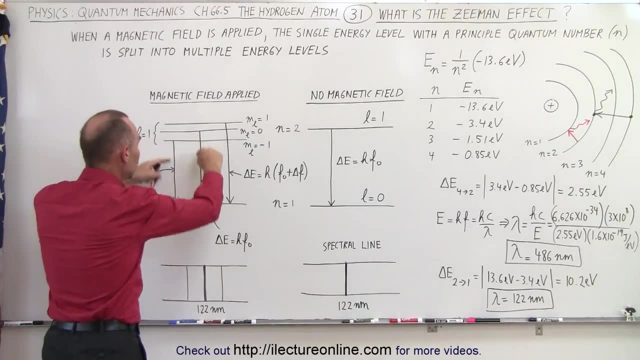 those three different orientations are slightly different. In other words, when we apply a magnetic field, we now have three different possible orientations for the angle momentum, and then the jumps of the electrons cause slightly different energy differences, which then would then be associated with the momentum of the orbital quantum number. 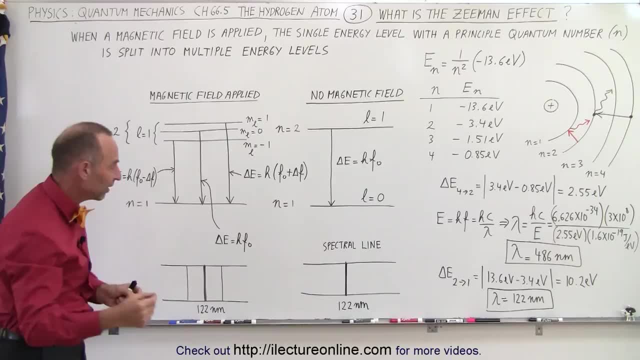 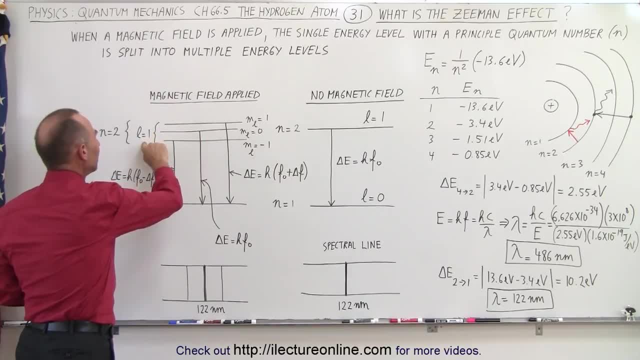 so that this would not split up, but for the l equals one or the n equals two level, where l equals one, the orbital quantum number equals one- there will be three different orbital magnetic quantum numbers associated with the three different levels that the electrons can be, which actually means they're associated with three different angle momentum directions, one that's 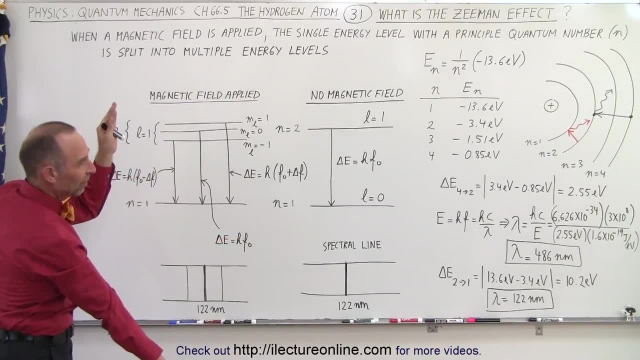 straight out relative to z-axis, one that's up here and one that one that's down there, and so therefore we have a split in the energy level, slight split causing a slight difference in the spectral line that we would see in the energy level, and so that's why we have a split in the 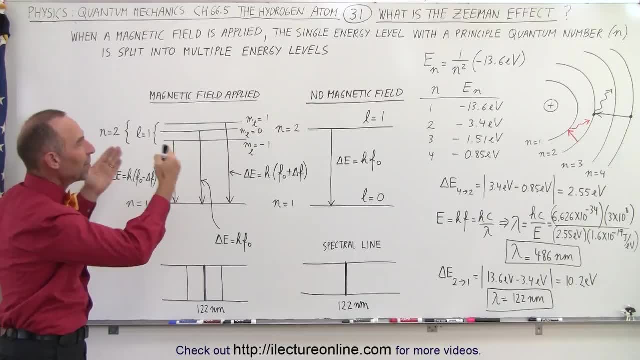 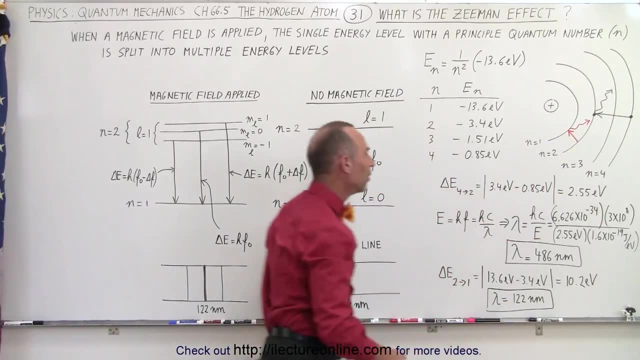 energy level that we would see and that discovery was then known as the z-man effect. you apply magnetic field and, all of a sudden, instead of having a single line associated with the jump from the second to the first level, we now have three different lines associated with the jump. 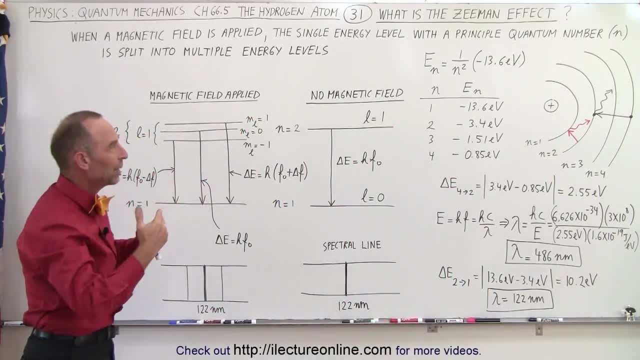 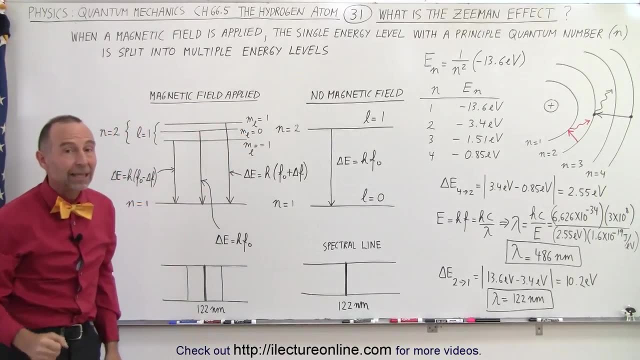 from the second to the first level, indicating that something was happening. there were more energy levels now, slightly different from the original energy level when a kinetic field was applied, and now we know that's due to the fact that the angle momentum has three different orientation within that specific energy level. when L equals 1..